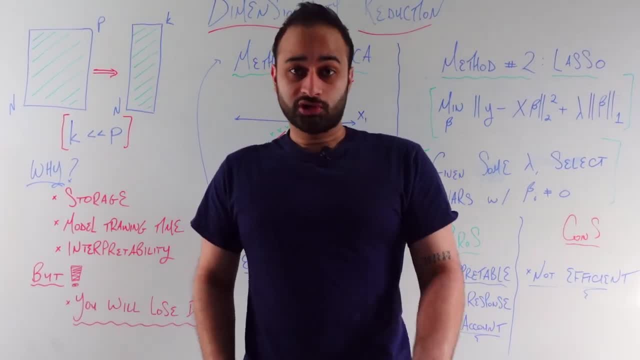 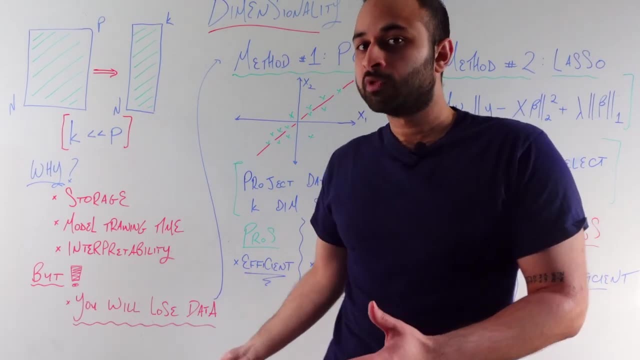 it could also be helpful for that, But it's very, very important to note in this video that when you do dimensionality reduction, however you do it, you're always going to be losing some data, And this is just intuitive. I don't think it requires a formal proof. You could do a formal proof, But 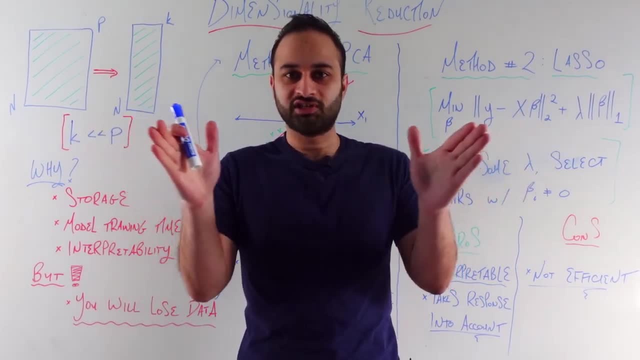 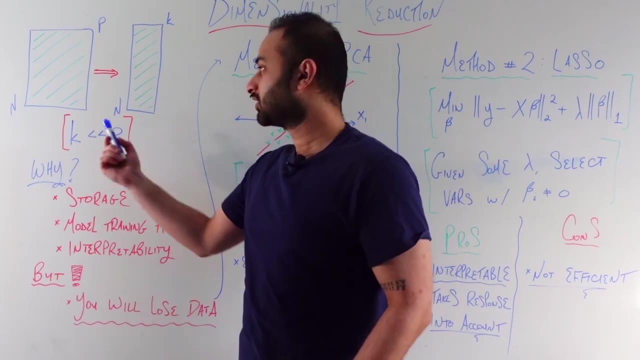 basically, if you're going from this much stuff and you're trying to press it into this much space, you literally just have less numbers, And so you can't capture all of the original dynamics in the original data set. And so the real goal of dimensionality reduction is not purely just give me less data, It's to compact. 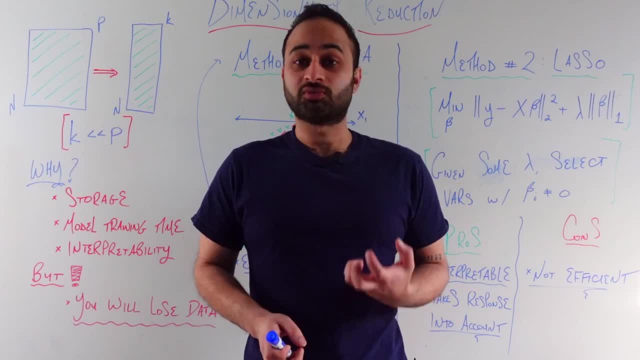 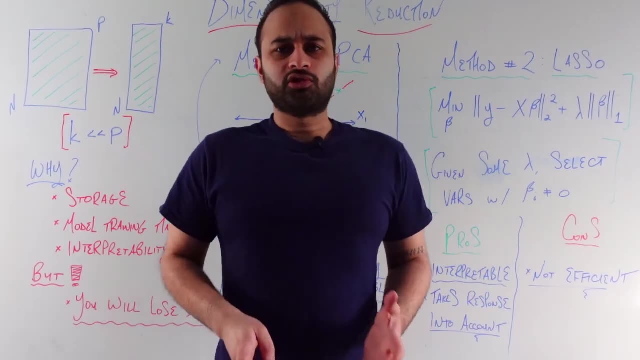 my data but lose as little of the valuable information as possible. So keep as much of the important stuff and throw away the stuff that's irrelevant. And so let's talk about two methods to do dimensionality reduction. There are many out there, but I want to go over two intro methods that you'll probably 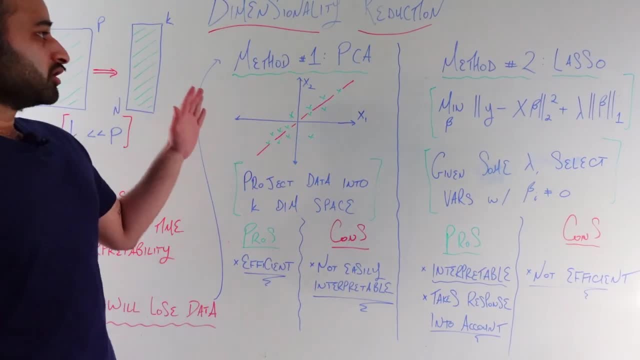 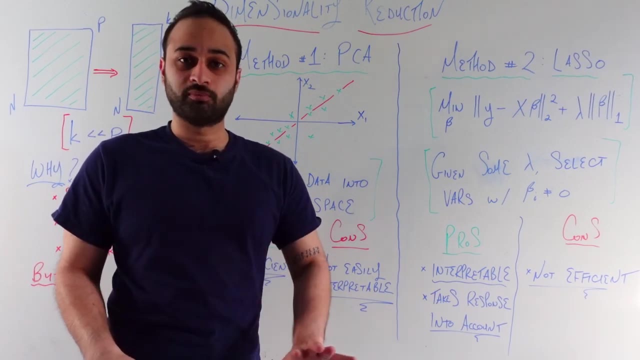 learn early on during your studies in machine learning. So the first one here is called PCA, or principal components analysis. Now, this is not a video where I'm going to go into all the depth of PCA. I have videos on that which I'll link in the description below. But just to remind you, here's a very 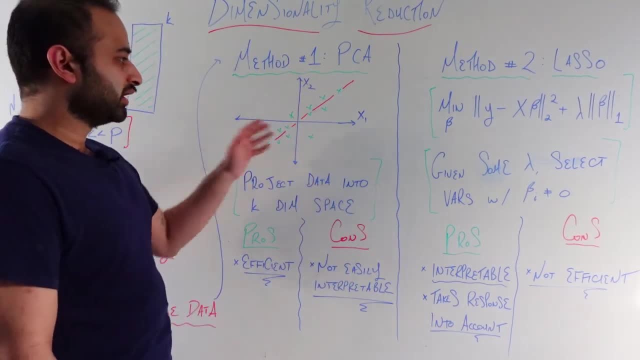 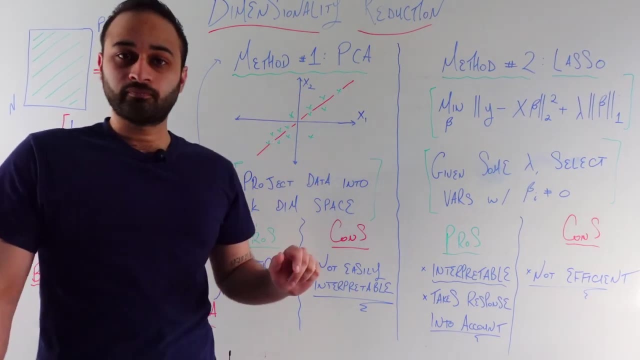 common picture you see during PCA. You might have some two dimensional data- x1, x2 coordinates- and all these green x's are your data points. You can see they more or less line up along this red line And so we project them into a lower dimensional space. In this case we're projecting our two. 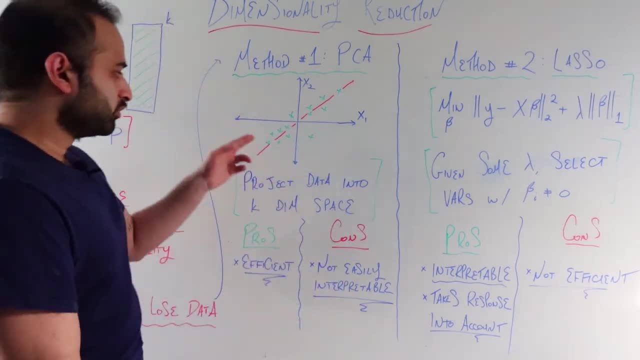 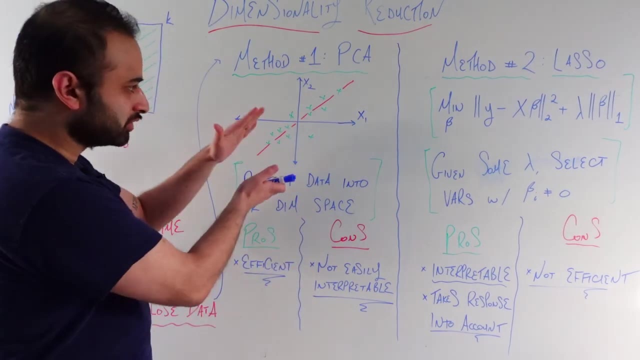 dimensional data into a one dimensional linear space. So you notice, when you project these green x's onto this red line, you're still going to be losing some data because the projections are going to be basically moving them into this one dimensional space, But because they already line up with the line pretty well. 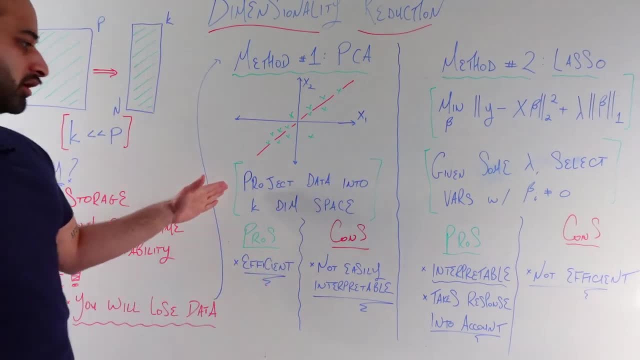 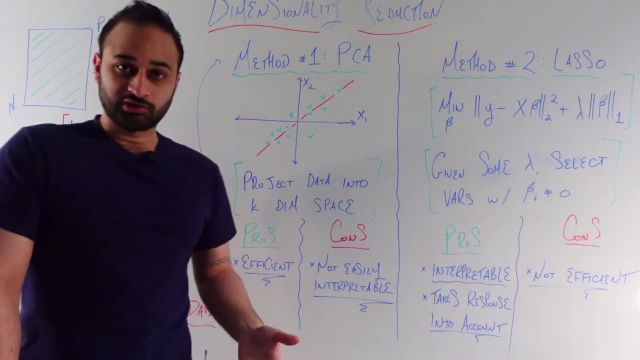 you're losing a very small amount of data, And so that's what's going on here: You're projecting your data into a k dimensional space where k is less than the original number of dimensions. Now, the pros of this is it's efficient. So, if you go through the entire process of PCA, it's basically built to compress your data. 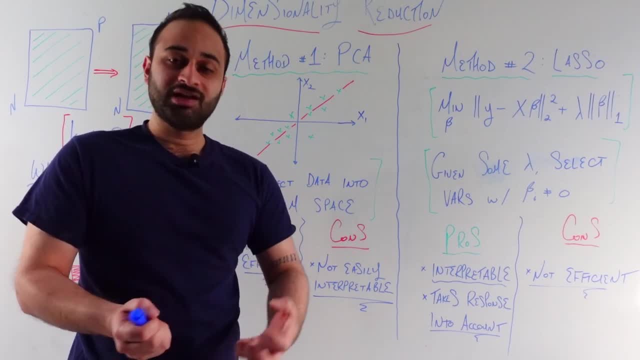 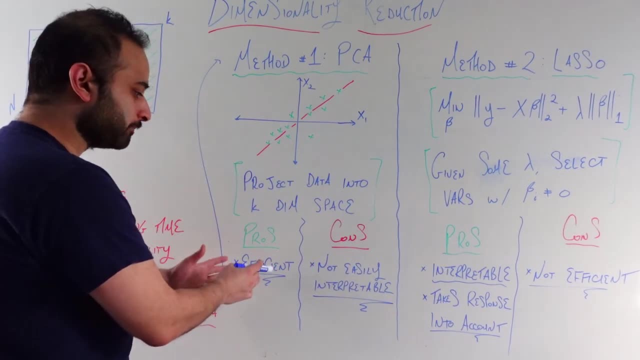 in such a way that you're going to be retaining as much of the variation in the original data set as possible. That's the entire goal of PCA, And so it's no surprise that it's doing that in an efficient way. But by being very efficient, you actually lose a lot in terms of interpretability. 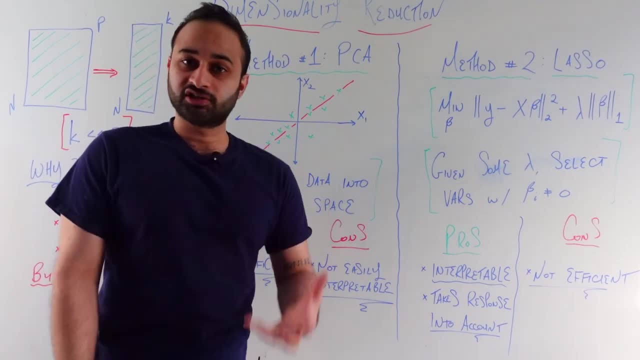 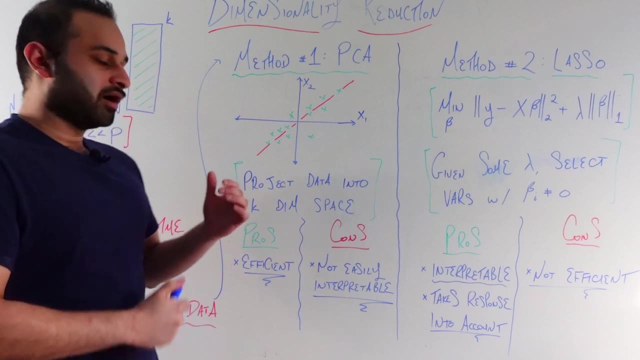 For example, to go a little bit deep into PCA for a second, you take the covariance matrix of your data. you find the eigenvectors of that. you project your data onto the eigenvectors of your covariance matrix- Obviously kind of a complex process- And so you lose a little bit of what's actually going on. 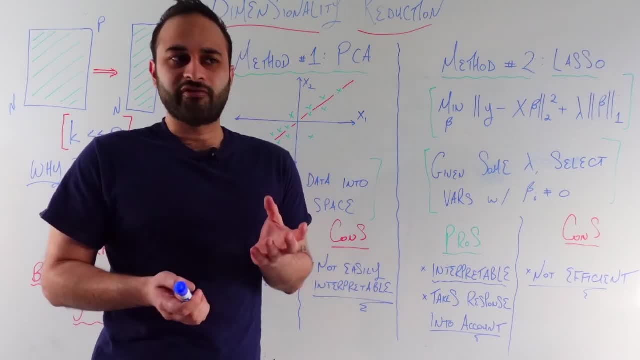 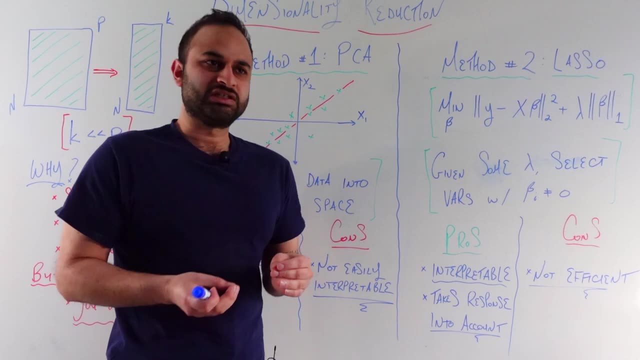 What does my transform data represent anymore? Because you're kind of now having to think about your transform data as coordinates, And so you have this new dimension, this new basis, basically new coordinate space, And so it's a little bit tricky- it's not impossible, but it's a little tricky- to map that back to your original features. 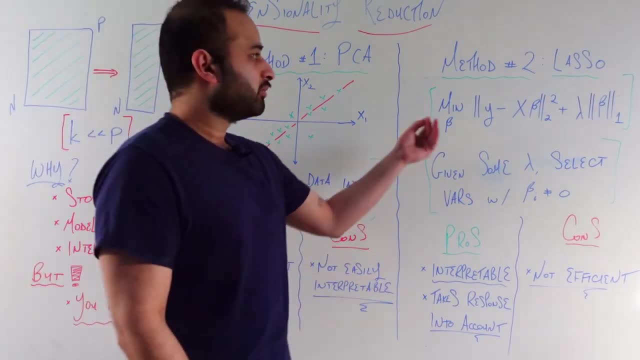 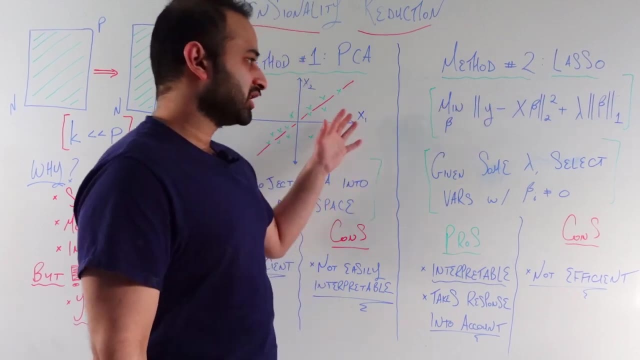 So it's important to note these pros and cons Now. the other major method I've seen in Intro machine learning courses to do dimensionality reduction is LASSO. So we've probably seen this formulation many, many times. But this is just a regularization of ordinary least squares. 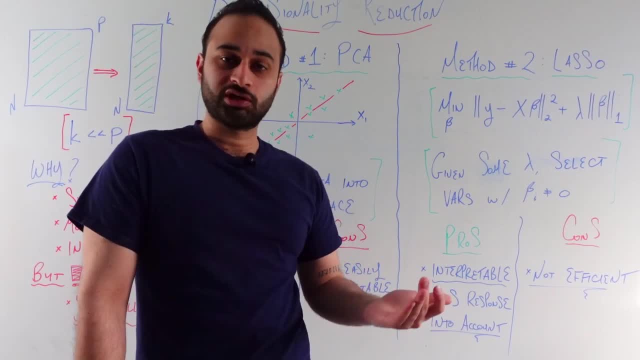 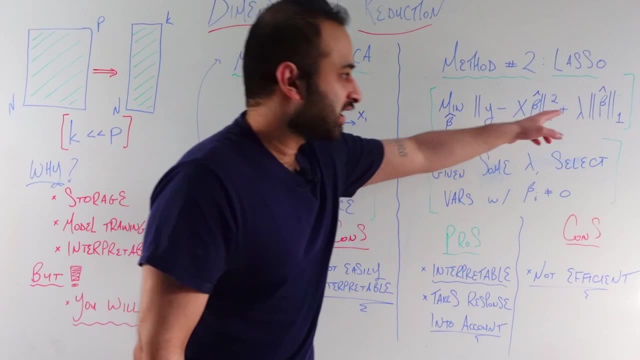 And we typically have this in two flavors. We have LASSO and Ridge and today's the LASSO formulation. So we're taking the true labels minus the predicted labels. we're taking the L2 norm of that, And then this extra term we tack on is for regularization. 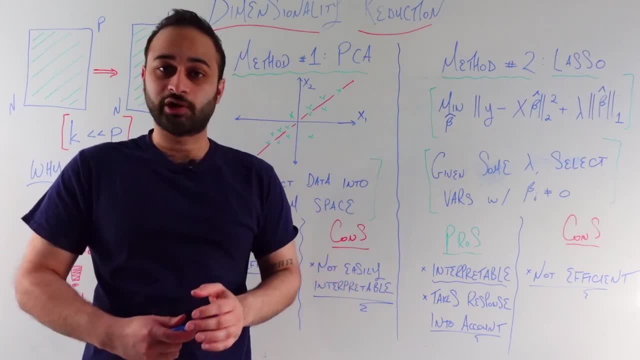 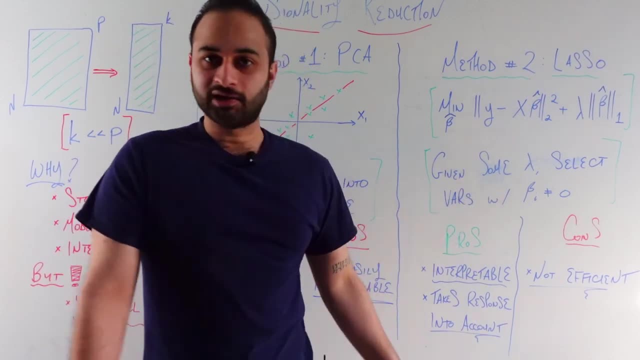 And when we have a L1 norm, as we do there, this is called lasso regularization, And the key feature of lasso regularization, as we know, is that it's going to send many of your beta- i's- to exactly zero. 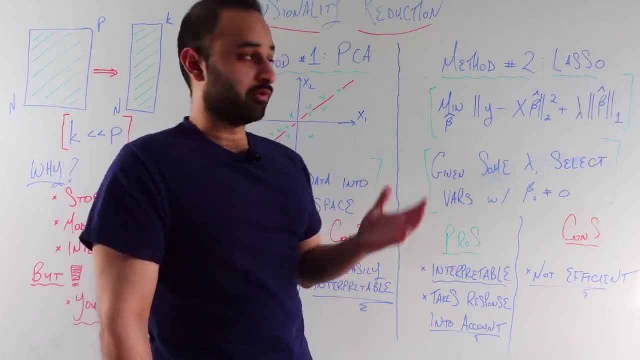 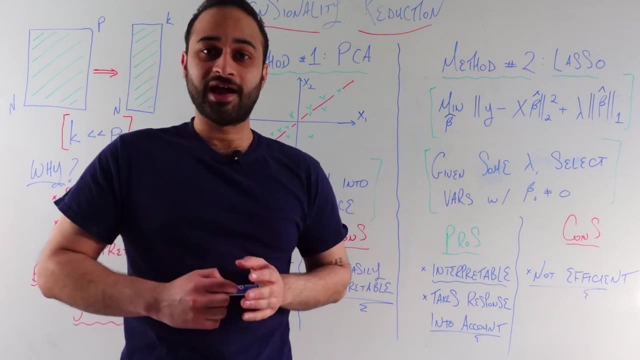 And so we can actually use this for feature selection, because we can run this. So let's say, we fix some kind of lambda which is a parameter, And then we can just pick the variables whose beta i's are not sent to exactly zero. 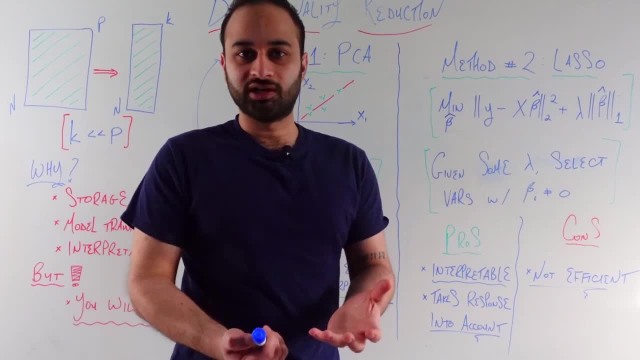 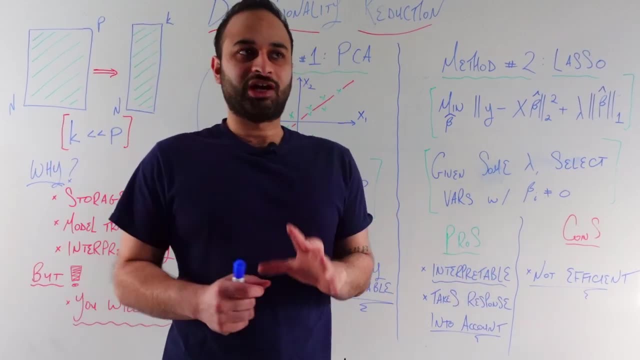 And in some sense, the model considers these as important or predictive of this target variable y. So the pros here are that this is interpretable. Notice, we're not projecting our data into any dimensional space. We're simply just eliminating columns that are not helpful in predicting this target variable y. 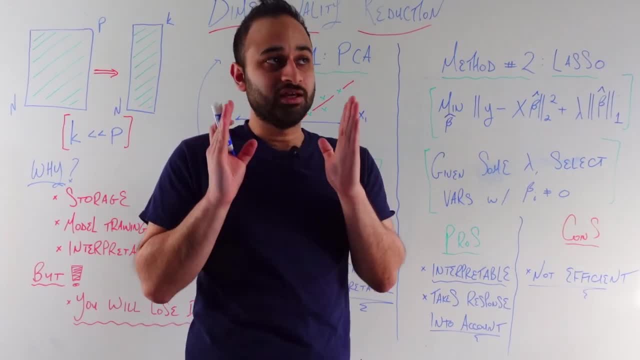 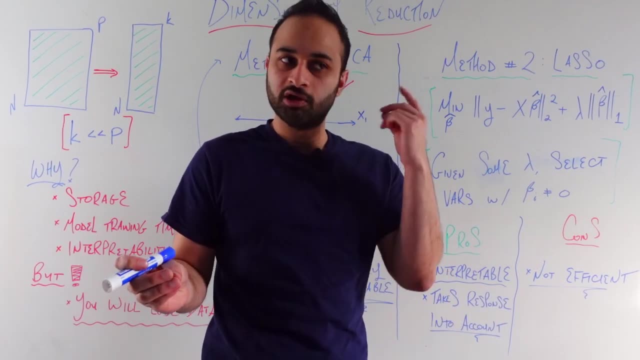 And so, at the end of the day, we have a smaller set of columns, but the key observation is that those columns are coming from the original data set itself. We're not transforming the features, So you can just say that, oh, this column was important. 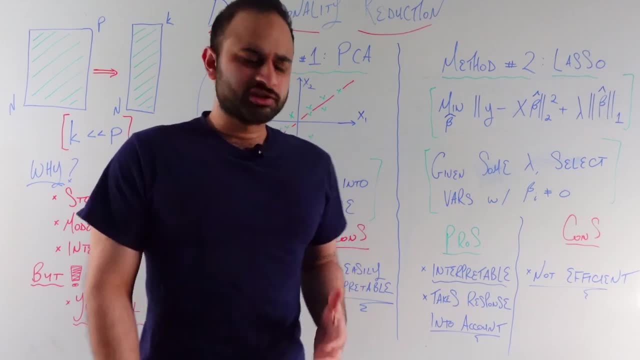 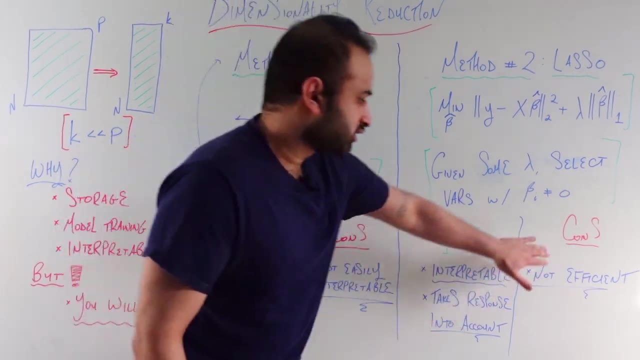 This column got thrown away, Easy to interpret, And the other kind of bonus is that it takes the response into account. Notice that y is explicitly taken into account here, which is not actually true for PCA, And of course the con here is that it's not going to be.